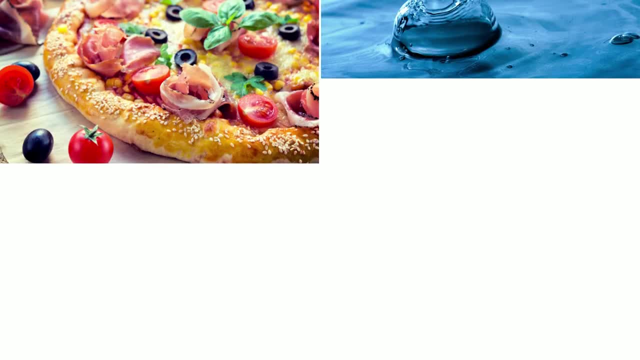 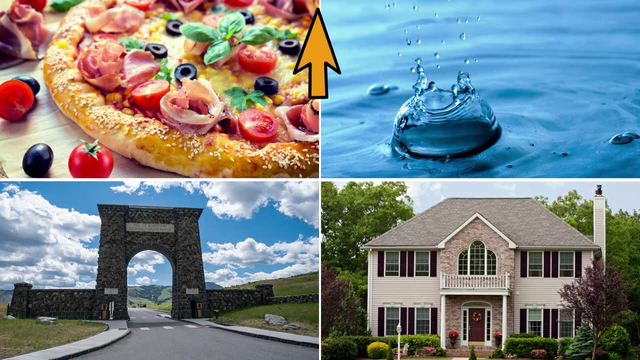 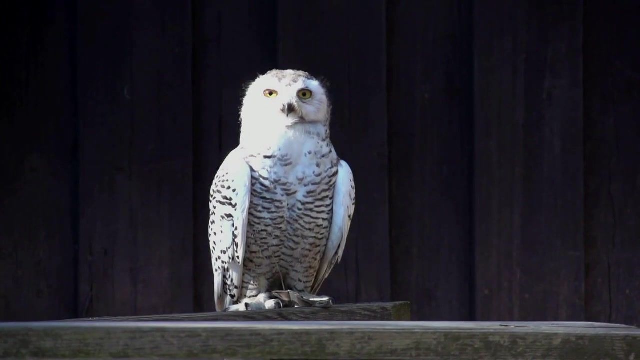 decrease If resources are available. a population will continue to grow until the resources will be used up. At this point, the caring capacity, which is the maximum number of individuals of one species that the environment can support, will be reached. For example, owls eat mice, small birds and other rodents in order to stay alive. 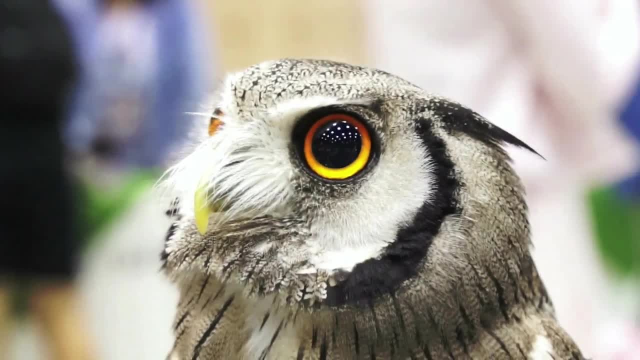 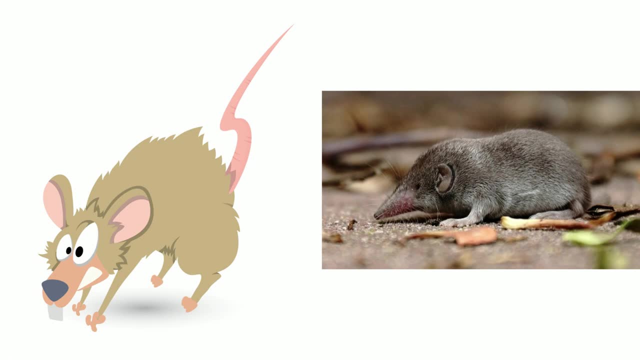 and, as a result, the caring capacity of the owls depends on the number of mice, birds and rodents available to eat. Owls also need trees to live in, and this also impacts the carrying capacity. The amount of food available for the owl and the amount of shelter are examples. 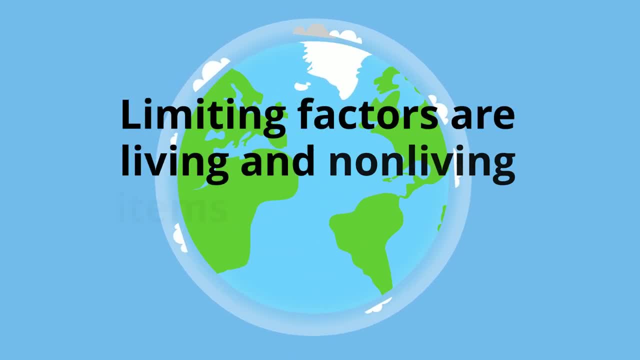 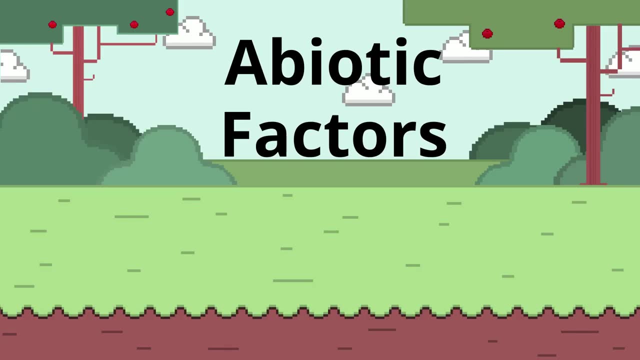 of limiting factors. Limiting factors are living and non-living items that restrict a population's size. Non-living parts of an environment are called abiotic factors. Examples include sunlight, temperature, water and rocks. Living factors are called biotic factors. Biotic factors will interact with other biotic factors. 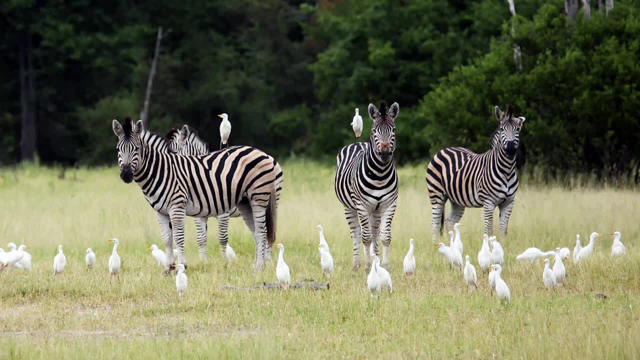 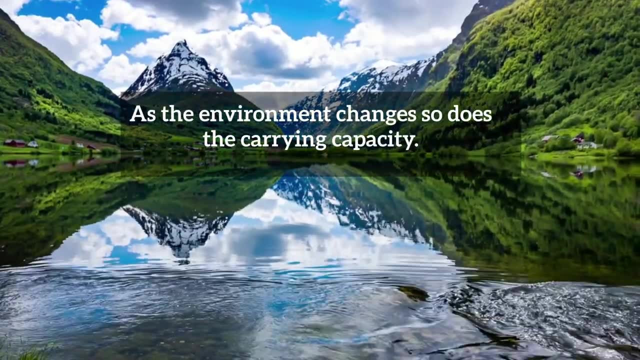 For example, zebras will eat grass, but lions will prey on the zebra. As the environment changes, so does the caring capacity. After a period of abundant rain, there may be extra plants available for insects and animals like zebras to eat. 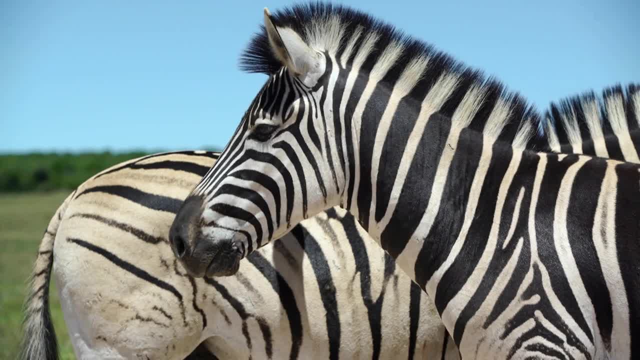 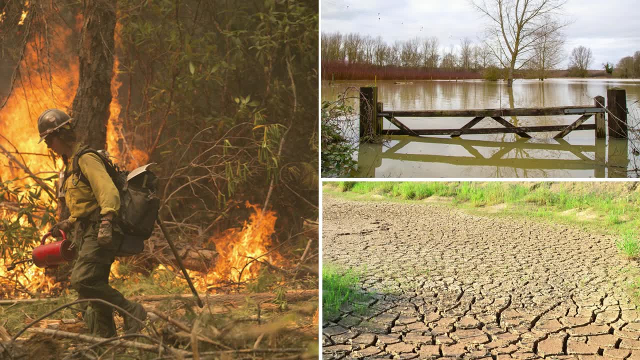 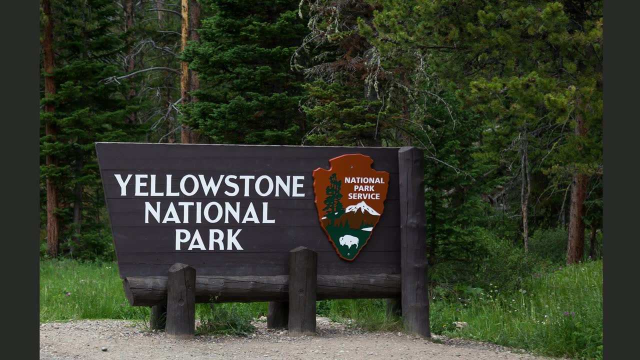 which will allow their population to grow. Conversely, natural disasters like fires, flooding or droughts can cause populations to decrease or even crash. Let's take a look at a real world example. Yellowstone National Park was established March 1, 1872. At this time, wolves were considered dangerous and were hunted. 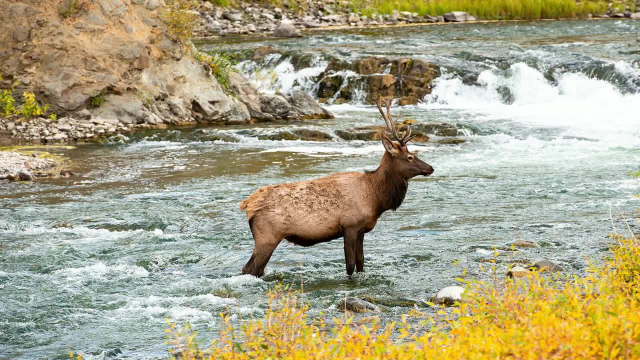 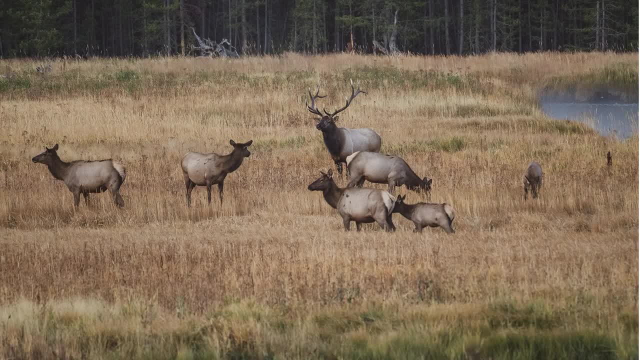 and driven completely out of the park. As a result, the elk population began to grow because one of the main predators was eliminated. On average, the population of elks in Yellowstone National Park was around 70,000.. The population of wolves in Yellowstone National Park was around. 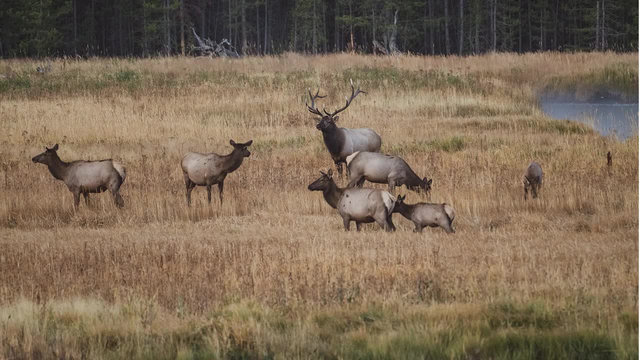 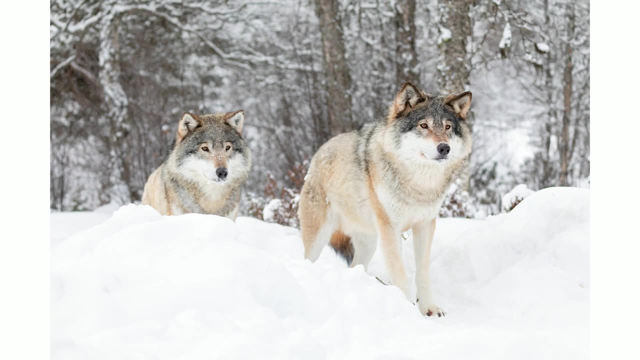 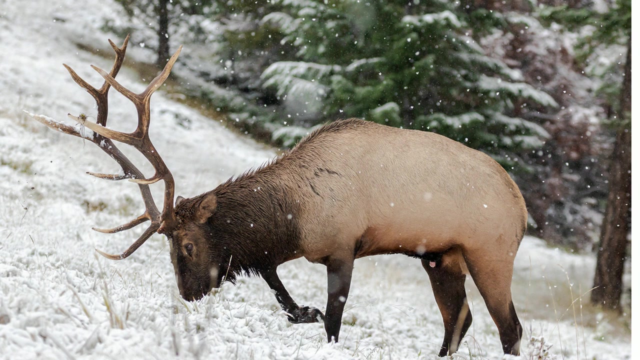 around 17,000.. On January 12, 1995, wolves were reintroduced in the park. As a result, the elk population fell below 10,000 in 2003 and in 2017, the number of elk was 5,349.